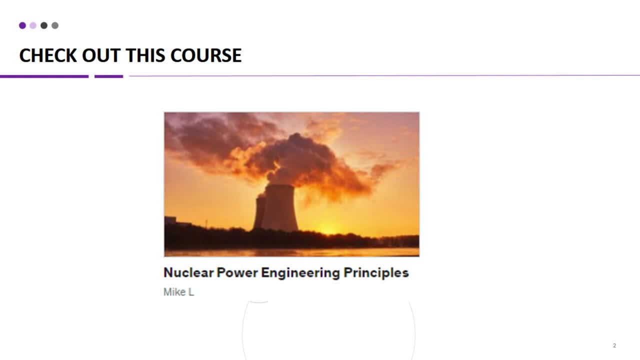 But hurry, as the course is still in progress. As this offer won't last long, Join us today and take the first step towards a successful career in nuclear power engineering. Enroll now in the Nuclear Power Engineering Principles course on Udemy and unlock your potential. 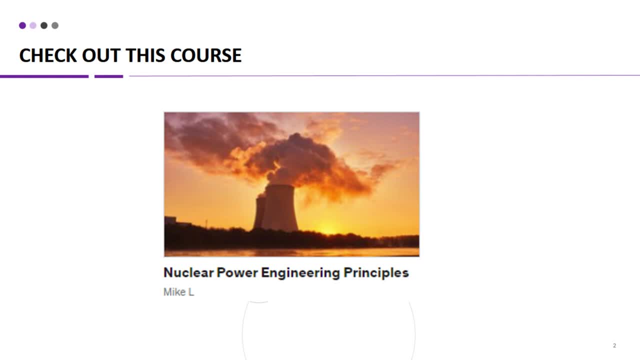 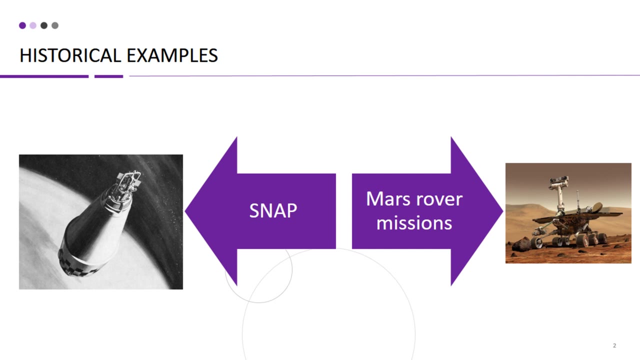 Don't wait and start your learning journey now. Now, if you're interested, the link to this course is provided in the video description below. Nuclear energy has a rich history of Powering Space Exploration Missions. One of the earliest examples is the SNAP Systems for Nuclear Auxiliary Power program, developed by the US Atomic Energy Commission in the 1960s. 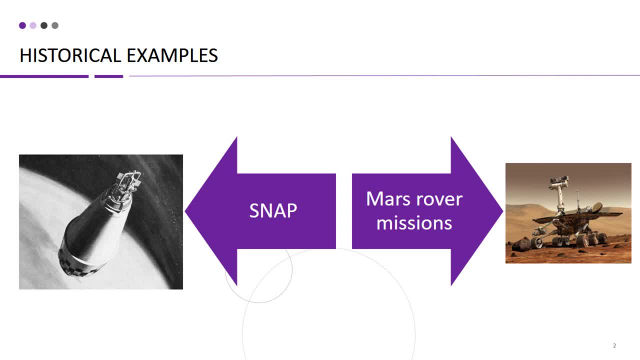 The SNAP program produced radioisotope thermoelectric generators- RTGs- that used the heat generated by the natural decay of radioactive isotopes such as plutonium-238, to generate electricity. RTGs have been used in several successful missions, including the Voyager spacecraft, which is still operational and sending back valuable data from interstellar space after more than 40 years in space. 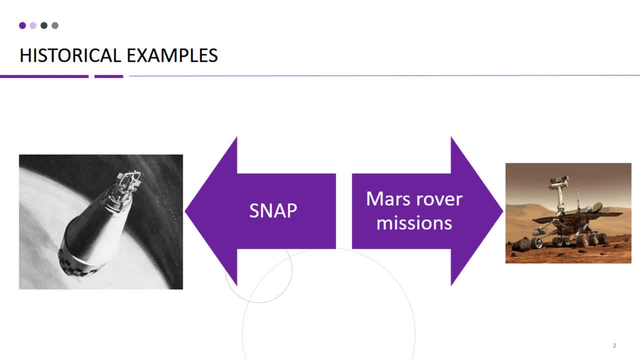 Another example is the Mars rover missions, such as Curiosity and Perseverance, which have used radioisotope power systems, RPs, to provide electricity for their scientific instruments and systems. Herpes have enabled these rovers to operate on the Martian surface for extended periods, despite the limited availability of solar energy in Mars's thin atmosphere. 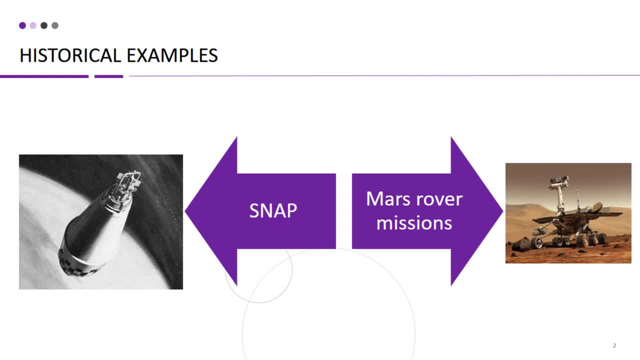 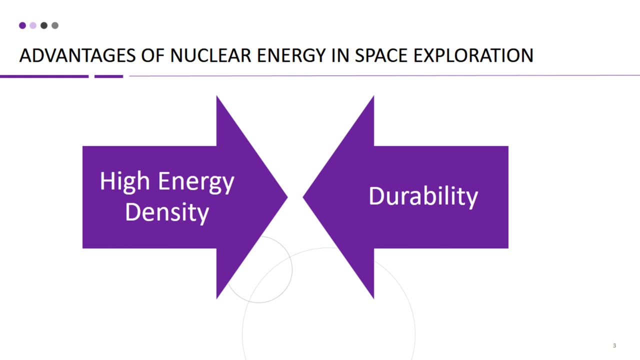 The use of nuclear energy has enabled these rovers to explore the red planet, collect valuable data and expand our understanding of Mars geology, climate and potential habitability. Nuclear energy offers several advantages for space exploration missions. One of the key advantages is its high energy density, which allows for the production of a significant amount of electricity in a small and lightweight package. 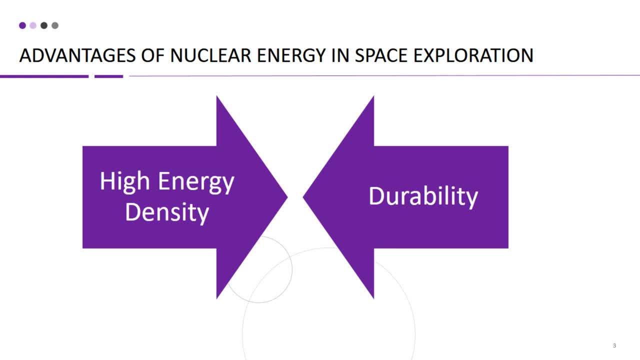 This is crucial for spacecraft, where every kilogram matters, as it determines the cost of launching the mission and the amount of payload that can be carried. Nuclear-powered systems can provide continuous power for extended periods, enabling long-duration missions and reducing the need for frequent battery replacements or reliance on solar energy, which may not be available in certain regions of space. 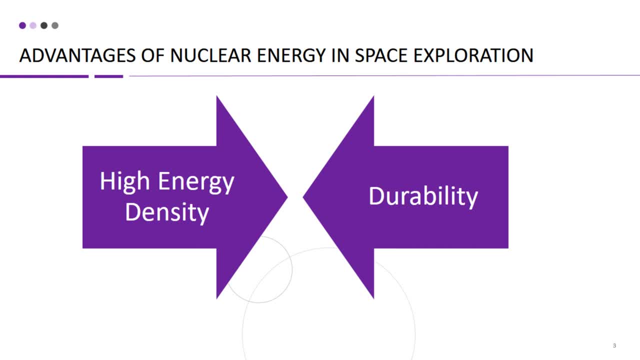 Another advantage is the durability of nuclear-powered systems. Radioactive isotopes such as plutonium-238, have long half-lives, which means they can continue to operate. They can also be used to produce heat and electricity for many years or even decades. 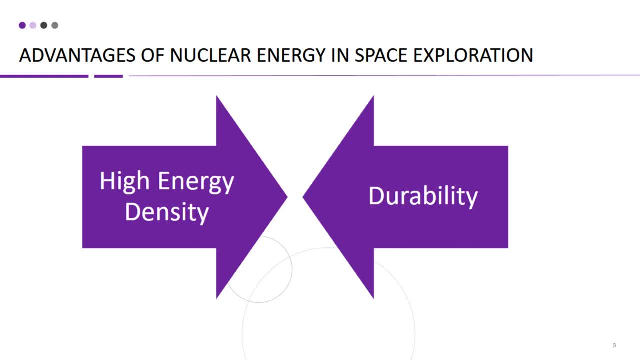 This makes them suitable for powering missions that require long-term operations, such as rovers or landers that need to survive in harsh environments for extended periods. Nuclear-powered systems are also relatively stable and can withstand extreme temperatures, radiation and other space hazards, making them reliable sources of power for space missions. 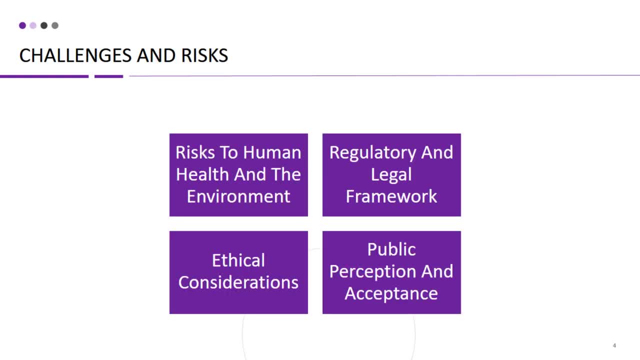 Despite the advantages of nuclear-powered systems, they can be used for long-duration missions. Nuclear energy for space exploration also poses challenges and risks. One of the primary challenges is the safety and security of nuclear-powered systems. Radioactive isotopes used in nuclear systems can pose risks to human health and the environment if not properly handled, stored and transported. 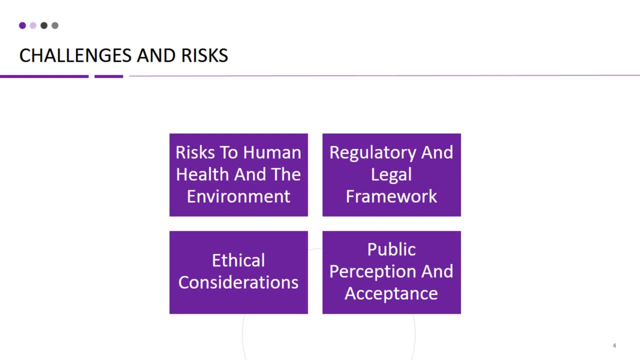 Ensuring the safe handling, transportation and storage of nuclear materials is critical to prevent any potential accidents in space. Radioactive isotopes are also very useful to prevent any potential accidents or releases of radioactive materials during space missions. Spacecraft powered by nuclear energy, such as RTGs or RPs, need to be designed and built to withstand the harsh conditions of space, including extreme temperatures, high levels of radiation and micrometeoroid impacts. 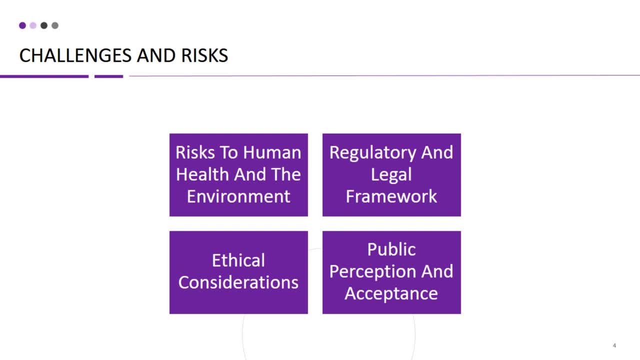 Any failure or damage to the nuclear-powered systems during launch, in-space operations or reentry can be a risk. An explosive burst of radiation or nuclear weapons or reentry could potentially result in the release of radioactive materials posing risks to the environment and public health. 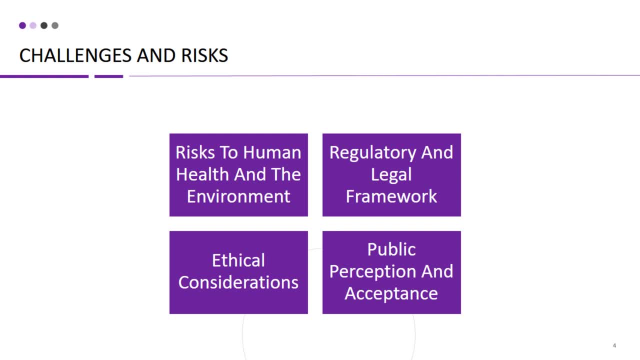 Another challenge is the regulatory and legal framework surrounding the use of nuclear energy in space exploration. International treaties, such as the Outer Space Treaty and the Treaty on the Nonproliferation of Nuclear Weapons, impose strict regulations on the use of nuclear materials in space to prevent their misuse or weaponization. 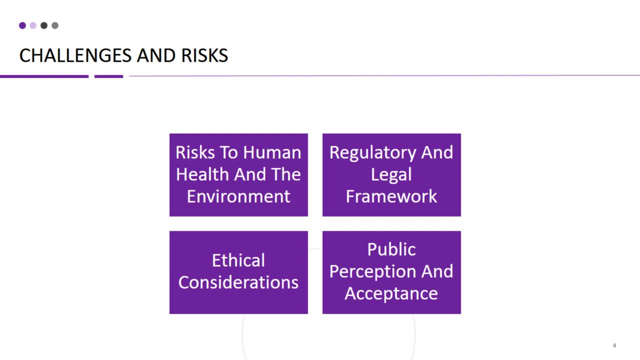 Like the United States, Continue to play the black card. Compliance with these treaties and other national and international regulations requires careful planning, coordination and cooperation among space-faring nations to ensure safe and responsible use of nuclear energy in space exploration. In addition, there are ethical considerations associated with the use of nuclear energy in space exploration. 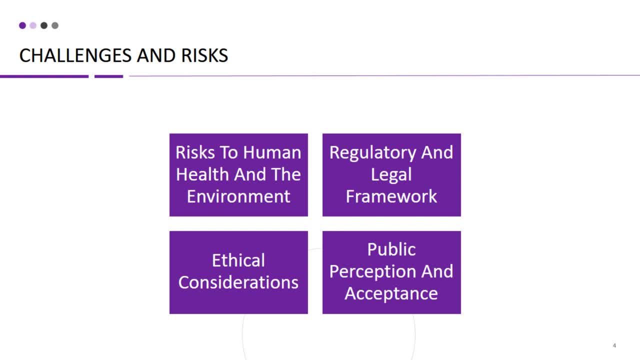 Some concerns include the potential for nuclear contamination of celestial bodies such as planets, moons or asteroids during exploration or resource extraction activities. Ensuring that nuclear-powered missions do not contaminate pristine environments and that any nuclear waste generated during space missions is properly managed and disposed of is a significant ethical consideration. 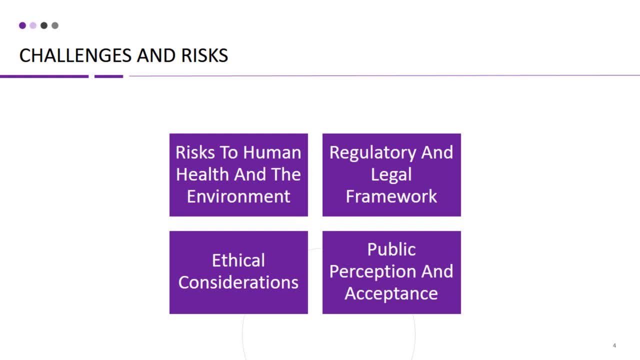 Furthermore, public perception and acceptance of nuclear energy is important. In addition, public perception and acceptance of nuclear energy in space exploration may also pose challenges. There may be concerns or fears related to the potential risks associated with nuclear materials in space, as well as their impact on Earth's environment and public health in case of accidents. 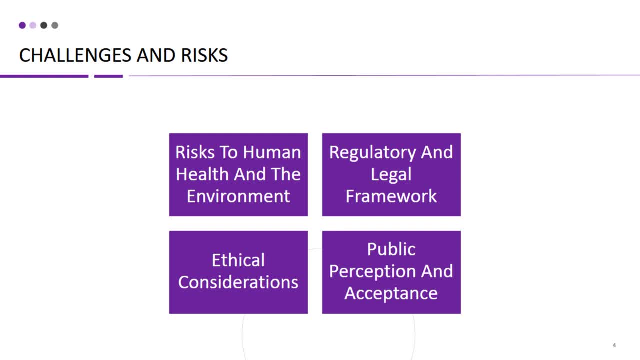 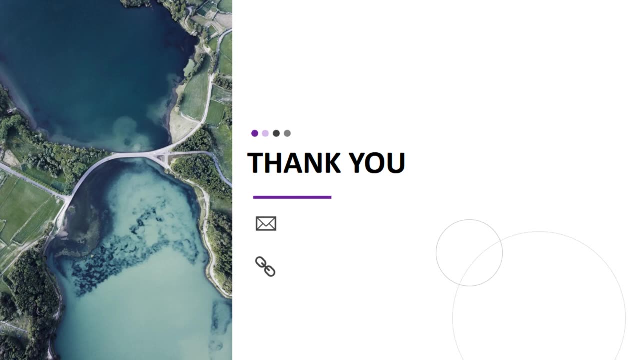 Educating the public and addressing any misconceptions or concerns related to the use of nuclear energy in space exploration would be important in gaining public support and acceptance for such missions. Thank you. In conclusion, nuclear energy has played and continues to play a vital role in space exploration, powering spacecraft and supporting long-duration missions. 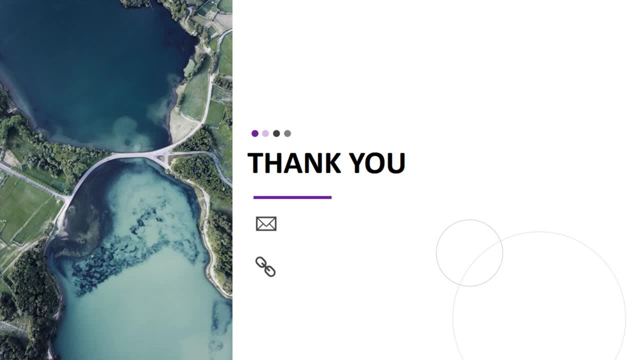 Its high energy density, durability and reliability make it an ideal source of power for space missions. However, there are also challenges and risks associated with the use of nuclear energy in space, including safety and security concerns, Regulatory and legal considerations, ethical considerations and public perception.